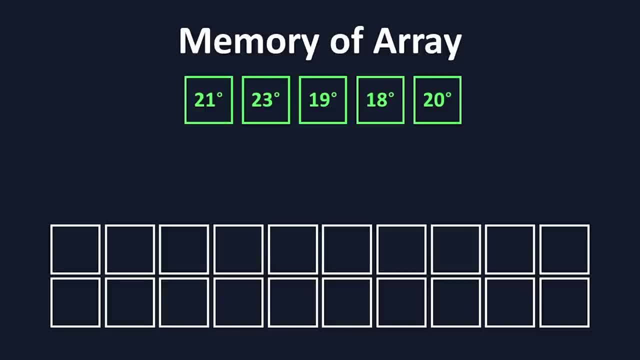 array from earlier. as an example, Arrays are stored in contiguous memory, which means each of the elements in the array are next to one another in memory. If a new element is added in the middle of the array, the entire array must shift down. But what would have happened if there was already? 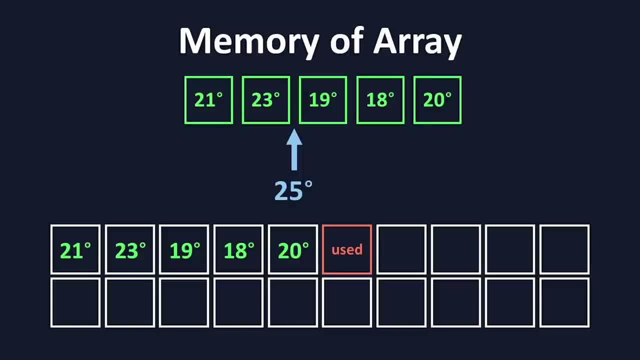 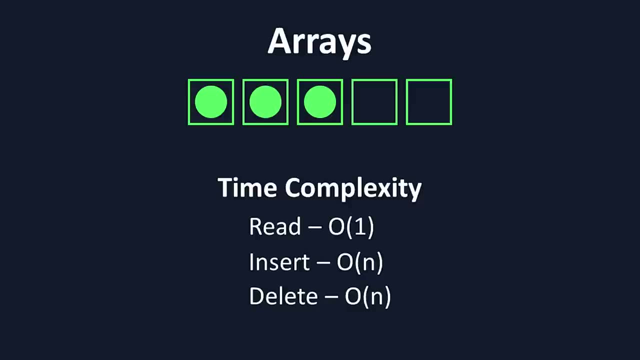 something in the next memory address To fit this new element in. now the array's memory will have to be reallocated to an entirely new space where all of the elements fit, While computers are not very efficient. So, to summarize: arrays are very good for reading elements, but can be a bit less. 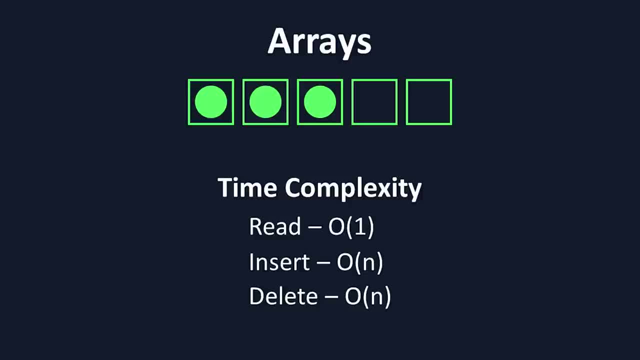 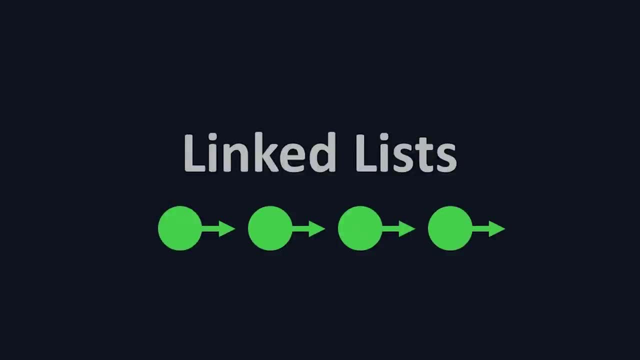 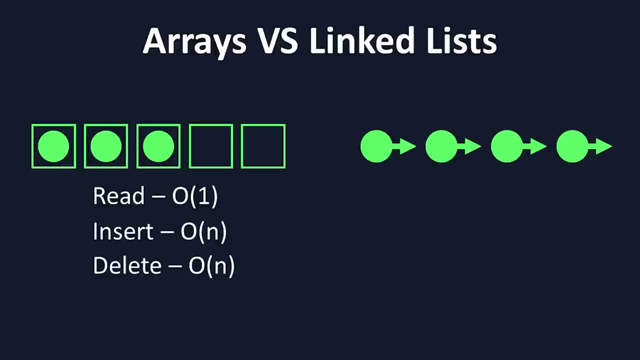 efficient when it comes to insertion or deletion. Now we'll take a look at a data structure that's the opposite. While arrays are fast at reading elements and a bit slower at inserting or deleting, linked lists are a bit slower at reading elements, but fast at inserting or deleting. 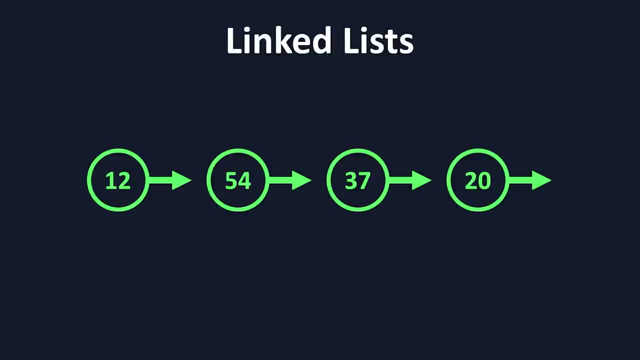 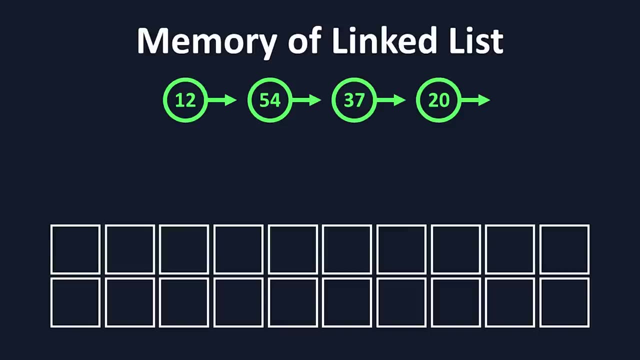 This is because linked lists are similar to arrays in that they also store ordered lists of data elements. However, a huge difference is in the way they are stored in memory. Each element of a linked list has what we call a pointer, which is basically the address of the next element of the list. 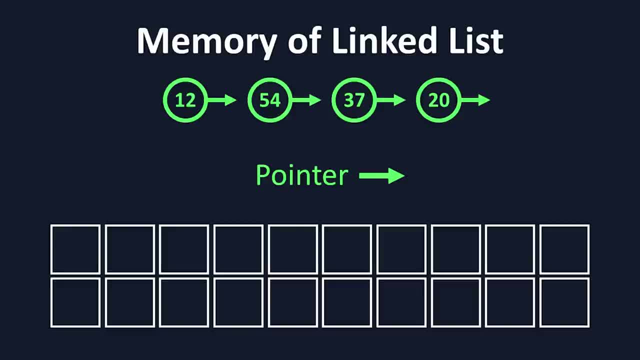 As a result, elements in a linked list do not have to be stored beside each other. You can store the next element in any location and the previous element will point to it if you want to find it. The advantage of this is that it solves our problem with array insertions and deletions. 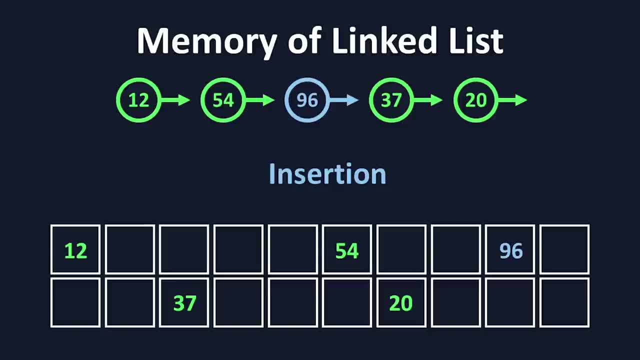 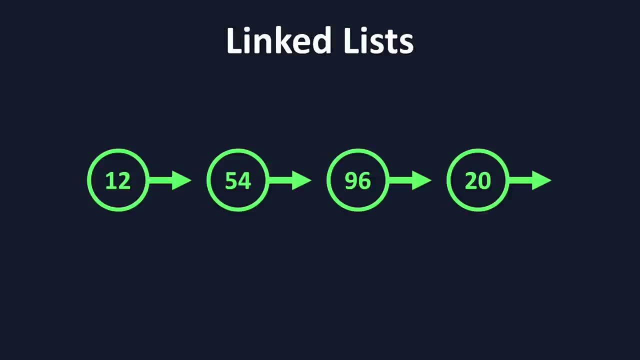 To add a new element, you find a free spot in memory for it and have the previous element point to it. To remove an element, you just delete the element and have the previous element point to the one ahead of the element you just deleted. The disadvantage of using linked lists is that 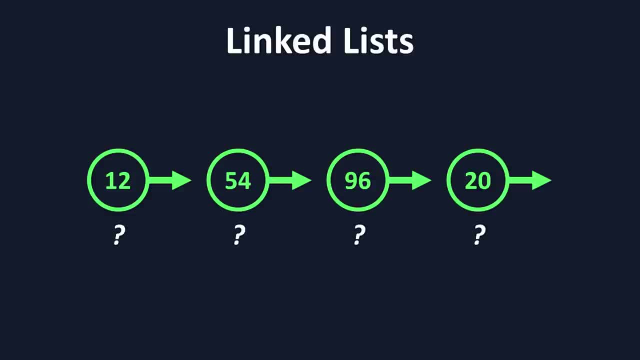 they do not have indexes as the elements are not stored right beside each other. This means that to find an element, we have to go through the list starting from the beginning. If we want the third element, we have to first look at the first element. 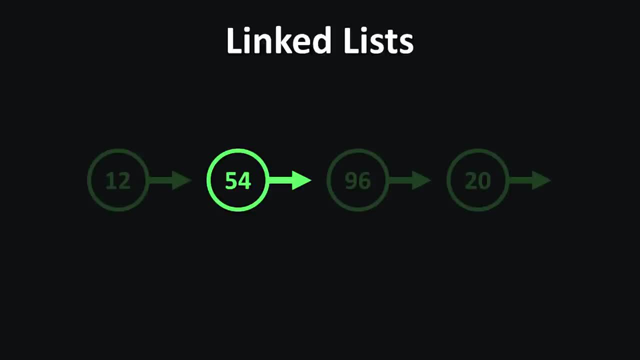 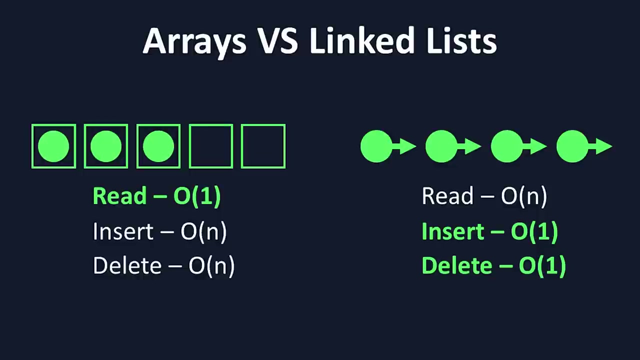 see where it points. go to the second, see where it points, and then we find the third element. If you think of a huge linked list, you can start to understand why it's not the fastest at reading. So to recap: arrays are faster when it comes to reading. linked lists are faster when it comes. 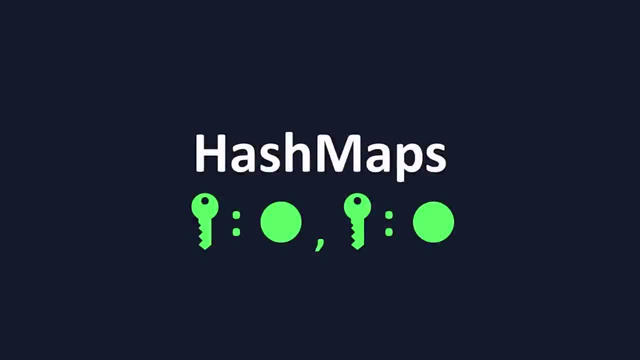 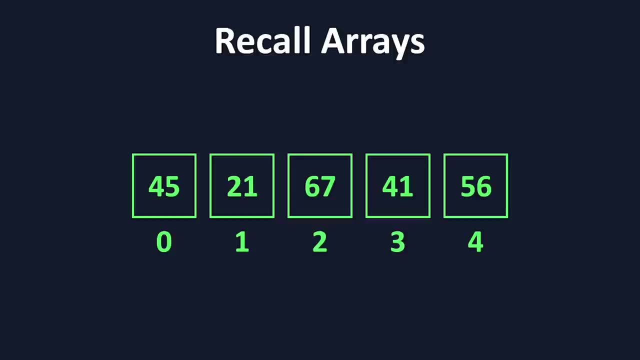 to inserting and deleting. Remember how arrays had values stored and for each value there was an index that numbered them. Well, hash maps are essentially the same thing, except that you can choose what the index is, which hash maps call a key. The key and its value are commonly known as key-value-pairs. 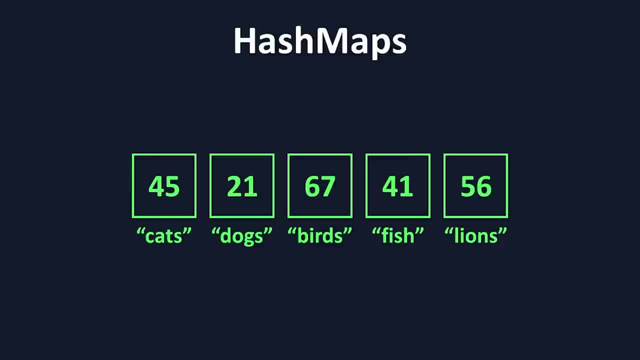 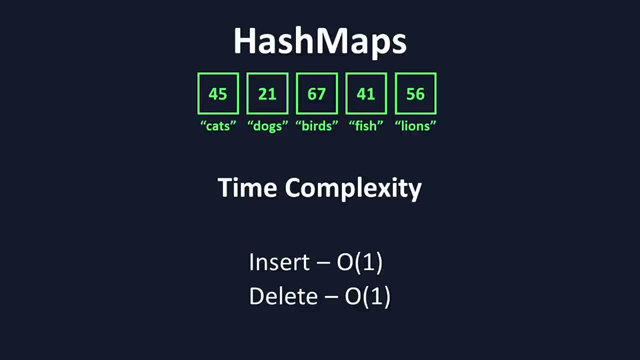 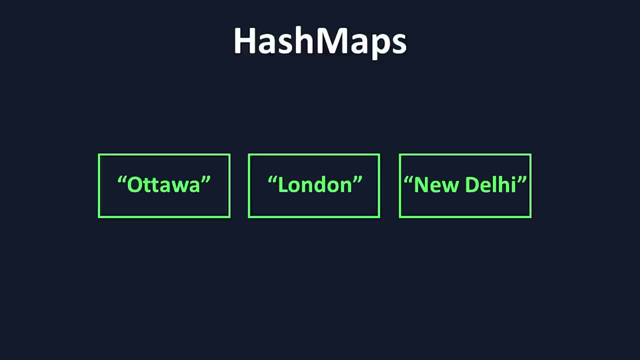 The other major difference between arrays and hash maps is that hash maps are unordered. Hash maps are fast for any value, both inserting and removing elements. But the real benefit to using HashMaps is their ability to search quickly. Let's say you wanted to store a list of capital cities. If we stored these in? 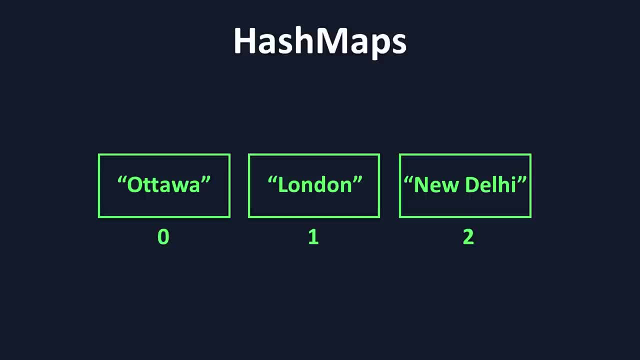 an array, we would have to know the index for each one to read it. But for a HashMap, if we make the keys countries, we can just look up the country to find the capital city associated with it. HashMaps go by a few different names. They are sometimes called hash tables. 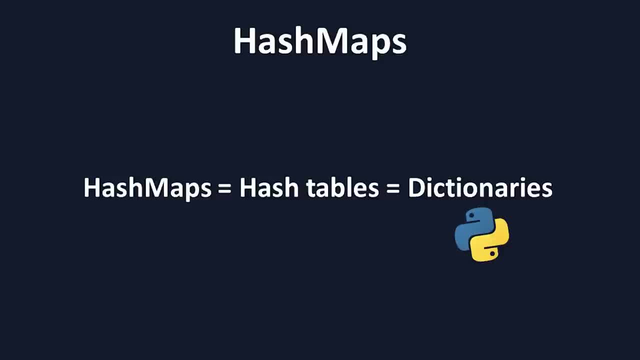 or, if you know Python, they're called dictionaries. For the purposes of this video, you can assume they're all the same thing. So if you know how to use dictionaries in Python, congratulations. you've actually been using HashMaps the entire time. 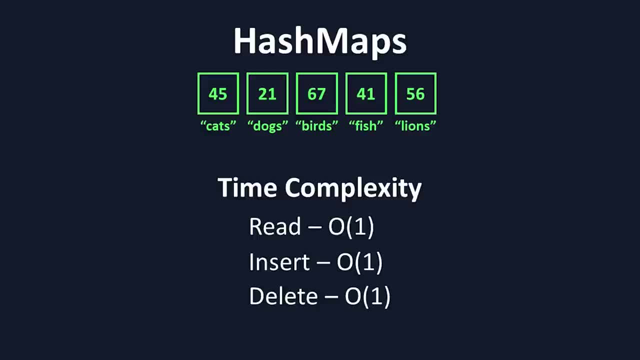 The way HashMaps work underneath the hood is really interesting, but a bit out of the scope of this video. I'll be making specific videos for all of the data structures, so we will cover HashMaps more in depth there. For now, just understand that they're all the same. 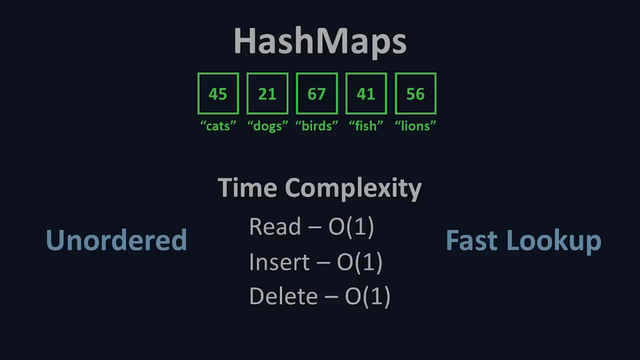 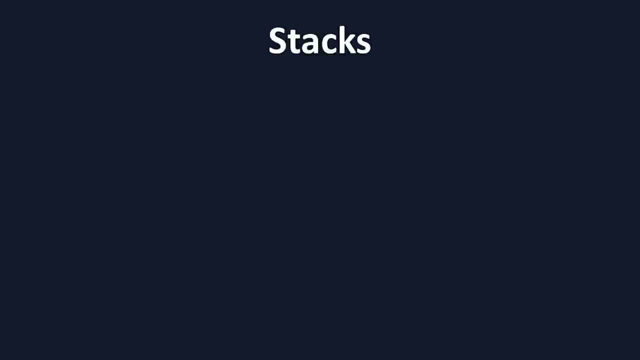 They're unordered and their custom keys allow for very quick searching. The most simple way to describe stacks is to think of a stack of plates or pancakes. The first plate goes on the bottom of the pile and the last plate goes on the top. 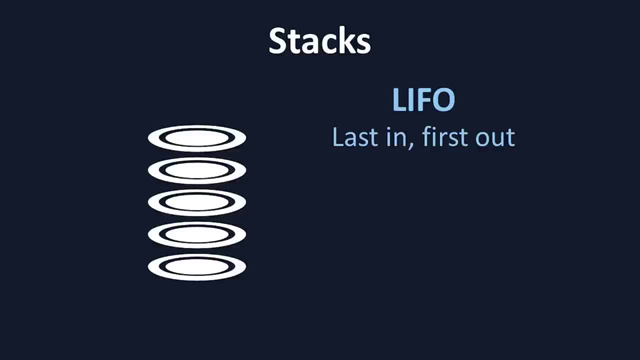 Stacks are called LIFO structures, which stands for Last In, First Out, because the last element in is like the last plate that goes on the top of the stack. When you go to grab a plate, the last plate on top will be the first one you take off. 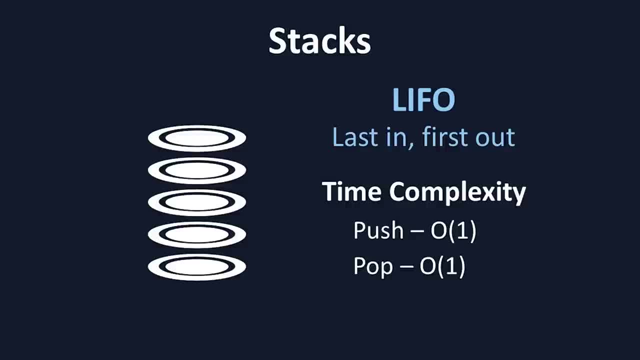 Stacks have three common operations, which are push, pop and peek. Pushing is when you add a new element to the top of the stack, Popping is when you remove the topmost element from the stack and peeking is when you're just taking a look at what the element at the top of the stack is. 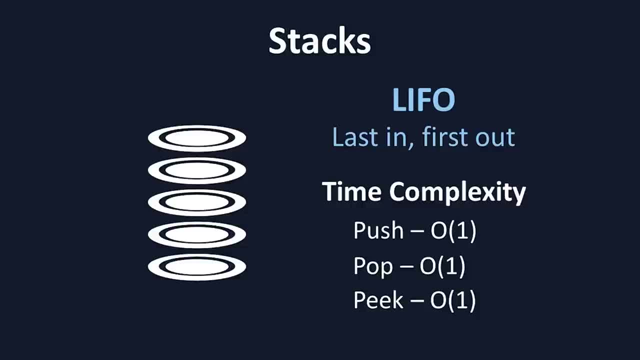 All of these are very fast, which is why stacks are optimal for certain problems. If you're wondering when stacks might be used, think of the pancake and plate examples, Any scenario that has a similar structure, where the last element in is the first element that should come out. stacks are likely a very good data structure to use. 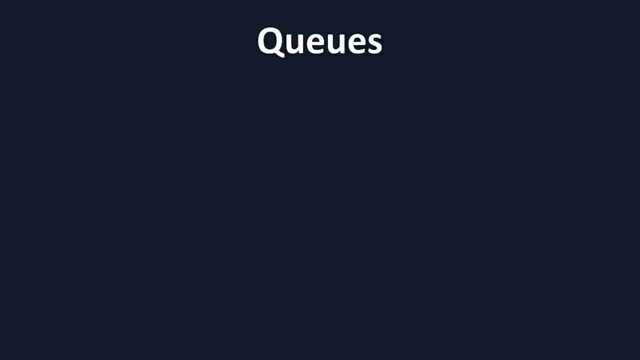 Queues are the opposites of stacks. The simplest way to think of a queue is like a lineup at a grocery store. The first person in the line will get serviced first, and every additional person who joins the line goes at the end. Queues are FIFO structures. 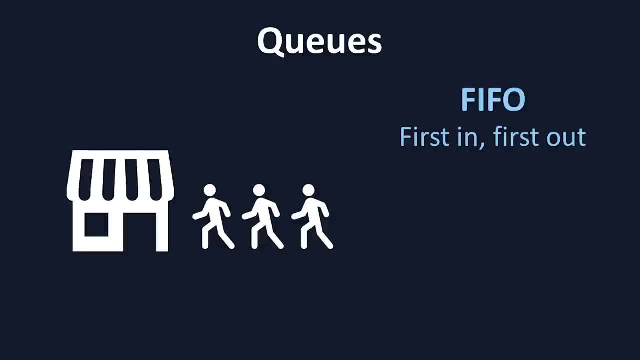 Which stands for first in, first out, because the first element in line is the first element to come out. Queues have very similar operations to stacks, which are called NQ, DQ and front. NQ is like push for a stack and is when a new element is added to the back of the queue. 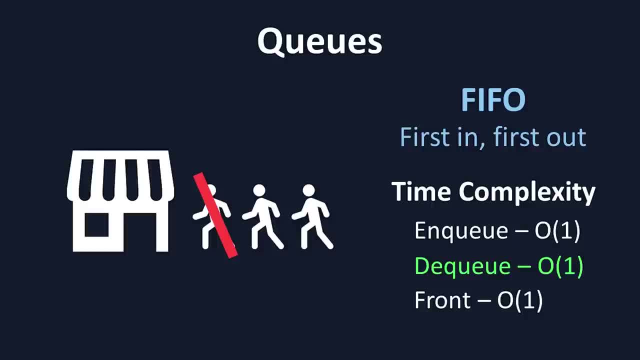 DQ is like pop for a stack, and is when the element on the front of the queue is removed, And front is like peek for a stack, and is when you take a look at the frontmost element in the queue. Queues are often more frequently used than stacks, especially in real-world programming. 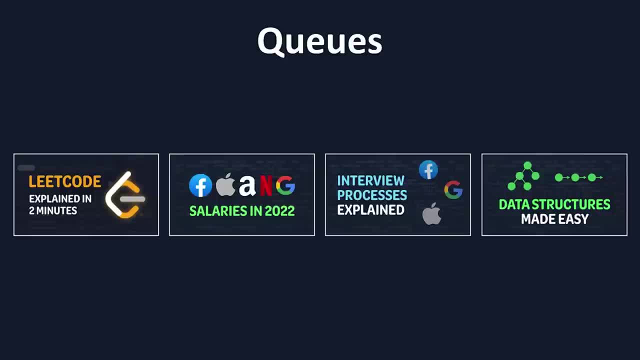 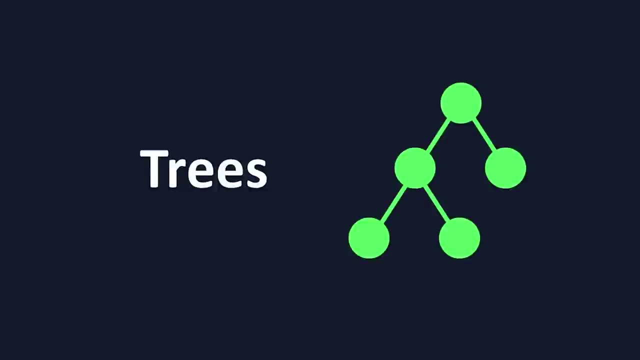 Think of something like YouTube playlists. When you start watching a playlist, you'll start with the video that was added first, and the last video you watch will be the final one that was added. Trees are a category of data structure that, as you might have guessed by the name, 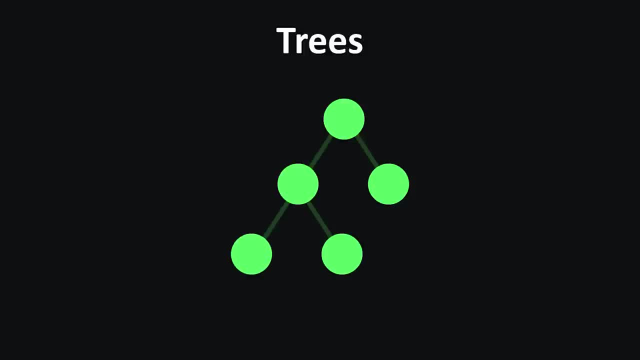 resemble trees. Trees have nodes which are connected to each other by edges. The first node in a tree is called the root node. Nodes have a parent-child direction. where one node is a parent node, that leads to another node which is a child node. 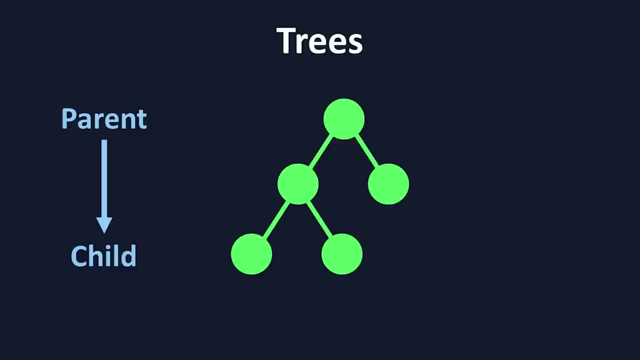 Sometimes people will refer to parent nodes as just regular nodes and the child nodes as leaves. There are tons of tree-based data structures, but in this video we'll be talking about binary trees and, in particular, binary search trees trees. A binary tree is a tree where the parent node has up to two children nodes. 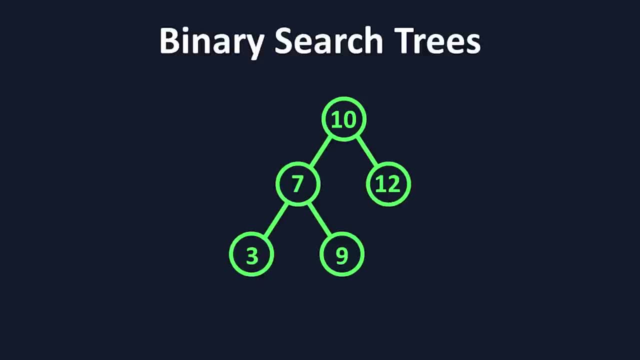 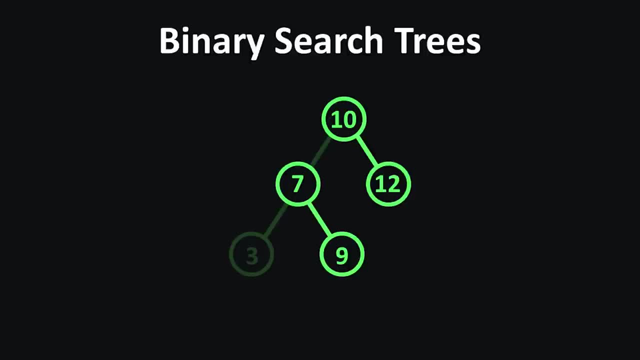 A binary search tree is a type of binary tree where all children nodes on the left are less than the parent node and all right children nodes are greater than the parent node. These binary search trees make it very easy to search through large amounts of ordered 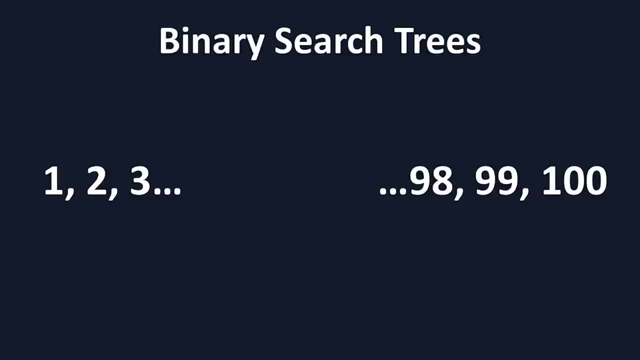 values. The classic example is to think of a number guessing game where one person thinks of a number between 1 and 100, and the other person has to guess. With each guess, they get told whether the correct number is higher or lower than their. 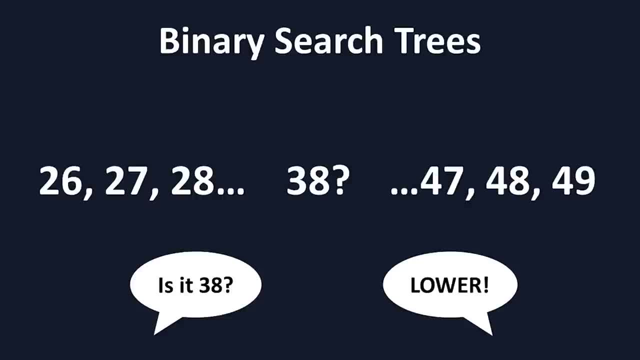 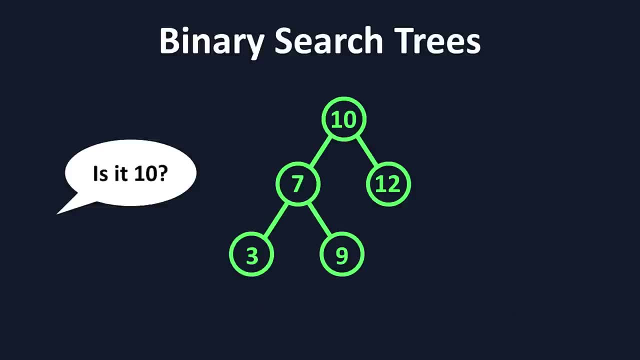 guess. The strategy is to always guess the middle number, because then you're eliminating the most amount possible each time. This is what a binary search tree does. We can eliminate a parent node and everything below it or above it and continue that process. 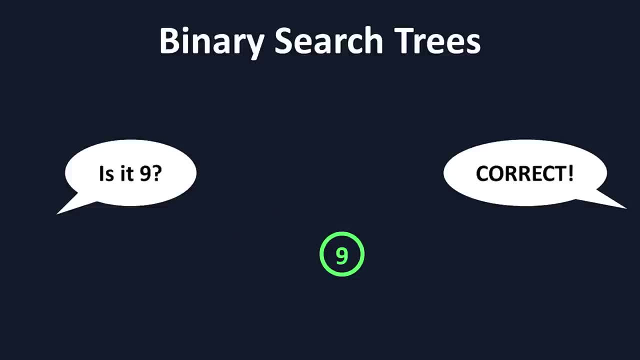 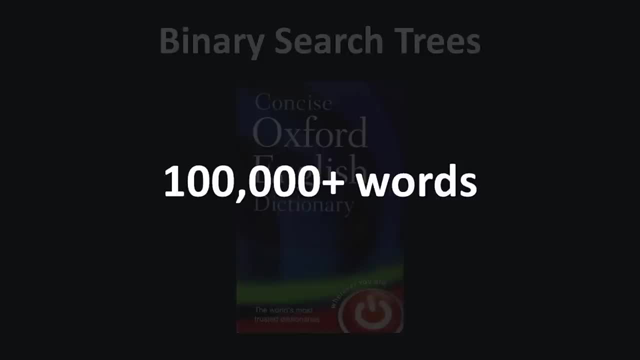 until we get to our correct number. This is not only useful for this game, though. A more practical example is to think of a digital dictionary. Dictionaries have over 100,000 words. If you give a computer a word and want it to give you back the definition, it would. 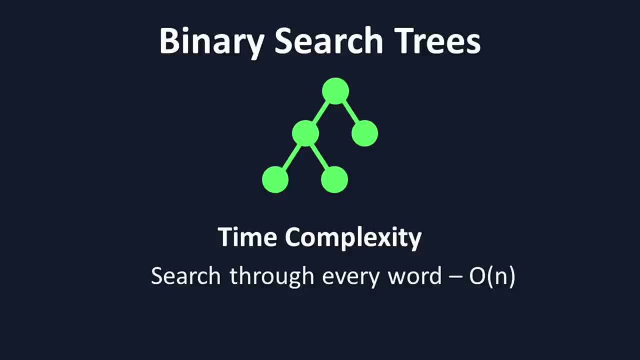 be incredibly slow for it to start at the beginning and search through every word until it finds the correct one. Instead, because the dictionary is sorted alphabetically, the computer is able to go right to the word in the middle of the dictionary and check if the target word comes before. 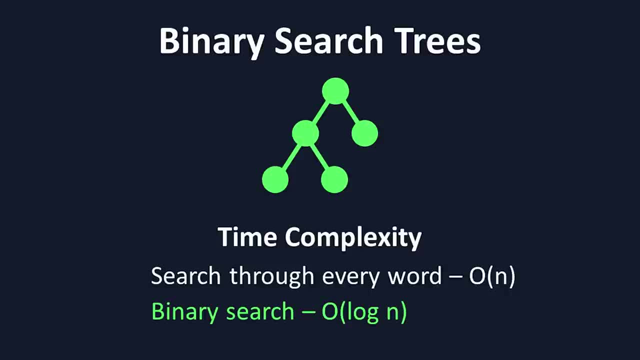 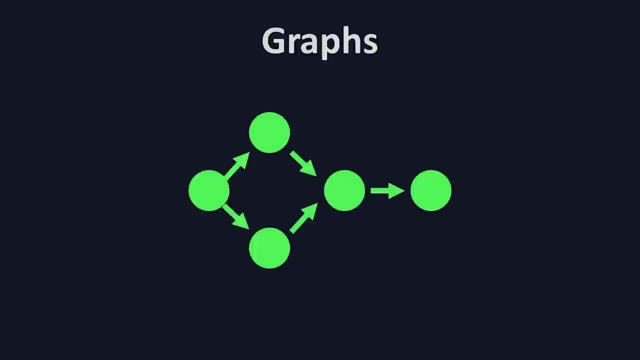 or after it, It continues sorting like this Until it reaches the word. There are tons of other tree-like structures like heaps and tris, but we'll be saving those for another video. Now onto our final data structure. Lastly, we have graphs. 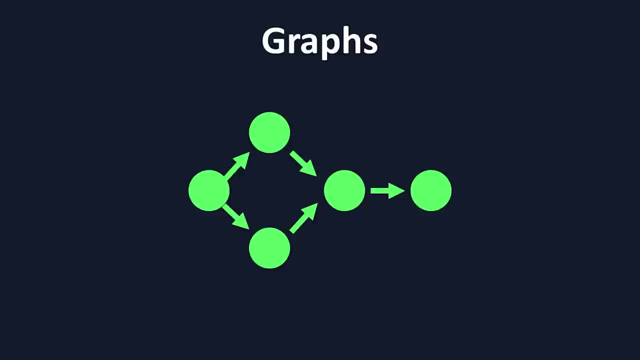 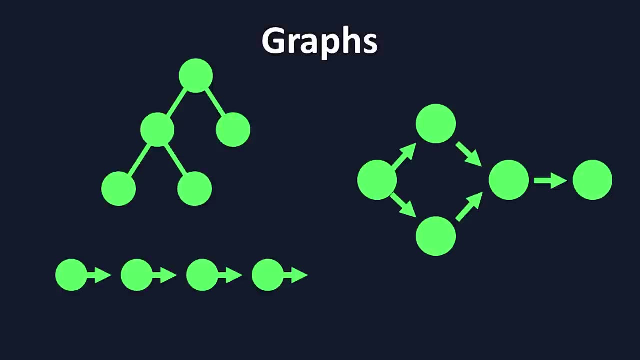 Graphs are basically models for a set of connections. Like trees, graphs are made up of nodes and edges. In fact, trees, and even linked lists to an extent, are technically just types. Graphs are basically models for a set of connections. 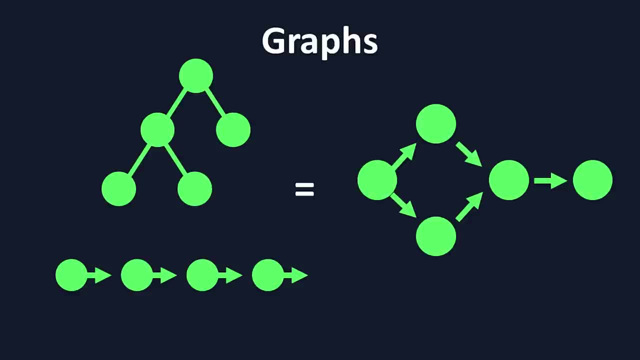 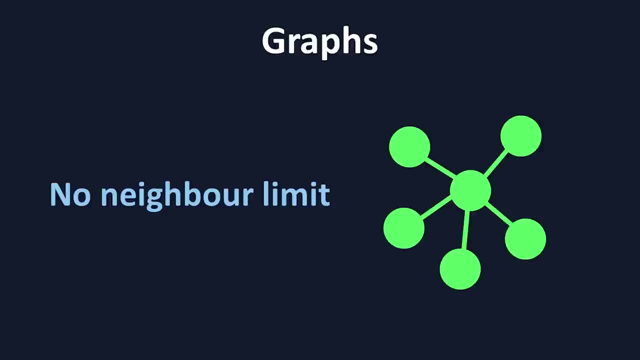 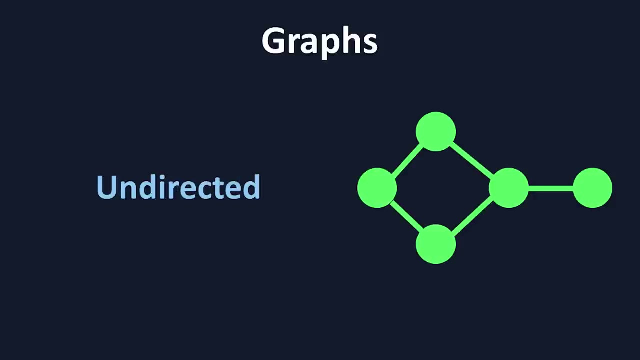 But graphs can get a lot more complicated than that. In a graph there are far less restrictions than with trees. Nodes can be connected to any amount of neighbors. Graphs can be directed where nodes point to other nodes, but they can also be undirected. 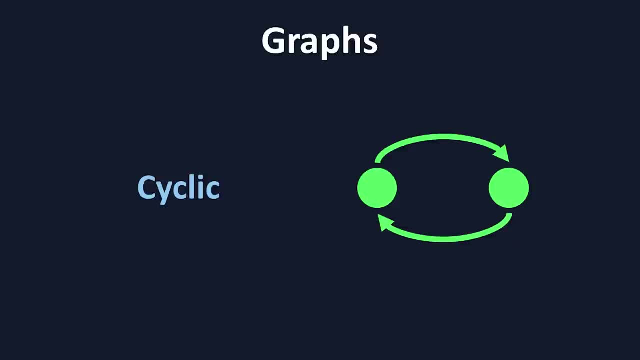 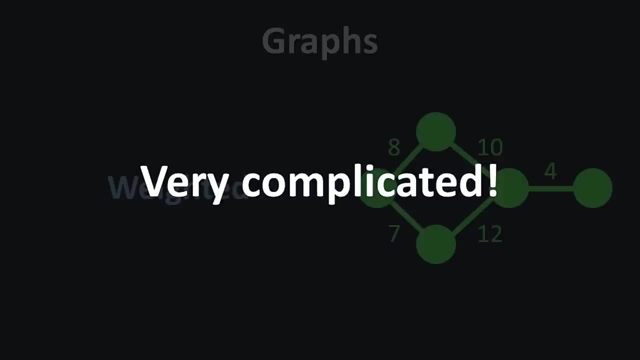 Some graphs have cycles where two nodes point to each other. The edges between nodes can also be weighted where the path has a value associated with it. As you can see, graphs are very complicated, Which is why many people consider them to be one of the hardest data structures to learn. 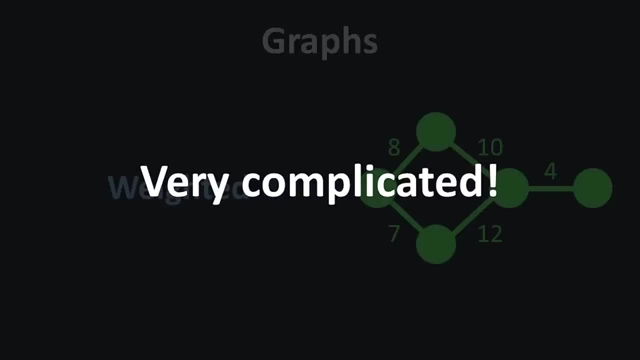 I'm going to make an entirely separate video dedicated to graphs, so we'll tackle the complexities in a little bit. For now, let's see an example where graphs are useful data structures. Imagine you're running errands and you have five different stores to visit. 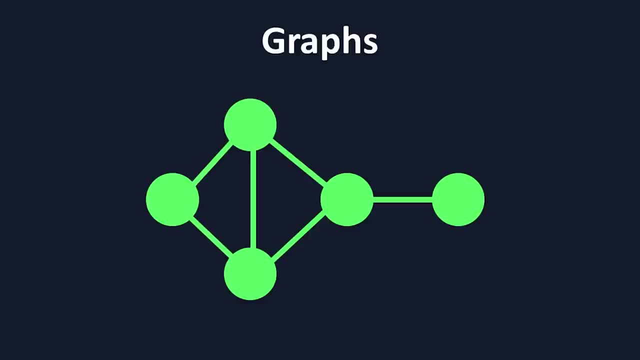 We can represent this as a graph where each store is a node and each edge has a distance. Using this data structure, we can develop an algorithm that allows us to calculate the shortest route between all five places. For a real-life example, think of Uber. 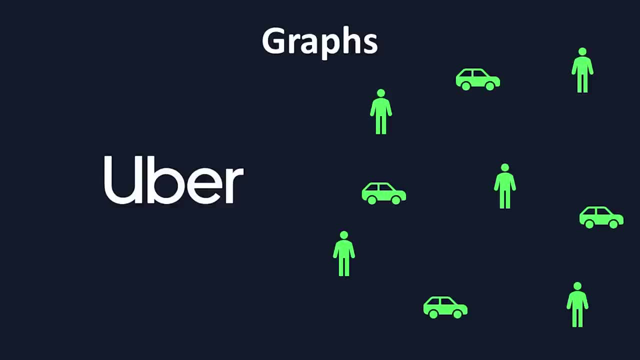 Every Uber driver and user could be seen as nodes, and the application is constantly trying to optimize so that the waiting time for each rider is as short as possible. There are endless applications to graphs, which is why they're such an important data structure to understand. 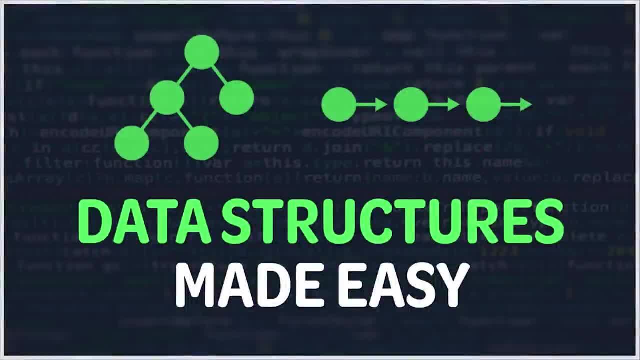 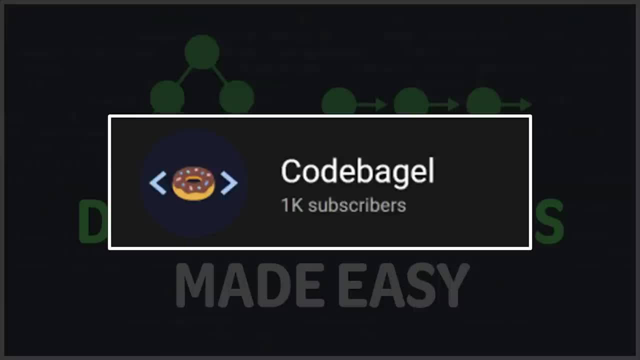 Thanks so much for watching. If you enjoyed this content on data structures and want to see more data structure videos, comment down below and leave a like on the video. I want to take a quick moment and express my gratitude to everyone for being so incredibly. 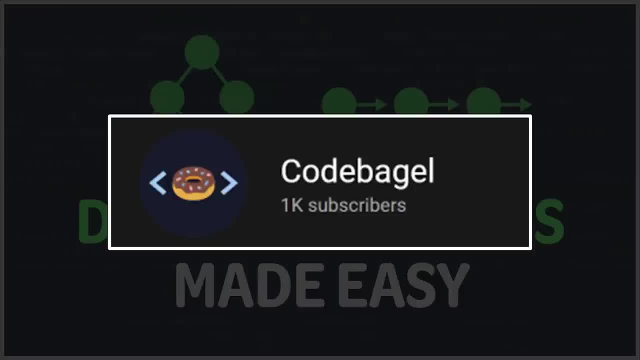 supportive so far and to celebrate hitting 1,000 subscribers. I started this channel just over a month ago and I've been super fortunate to have found 1,000 amazing people who have been willing to take a chance on my small YouTube channel. 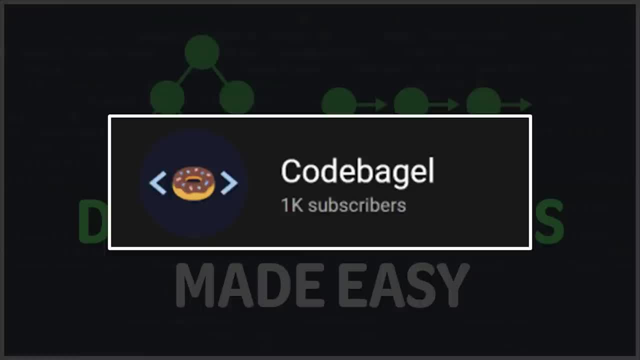 I never thought I'd be able to hit 100 subscribers in this time, Let alone 1,000. So I'm just so thankful that all of you guys have been so supportive. I promise I'll do my absolute best to continue increasing the quality and quantity of content. 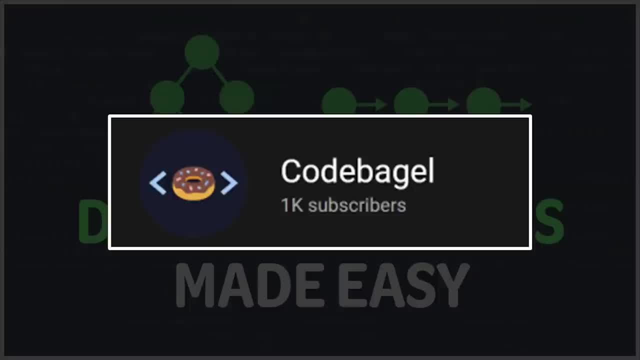 as much as I can. Thank you and 10,000,. here we come.